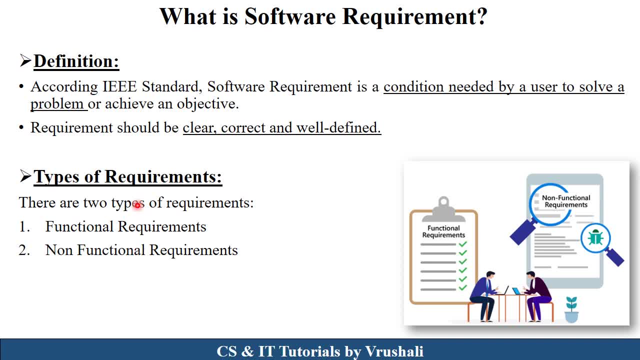 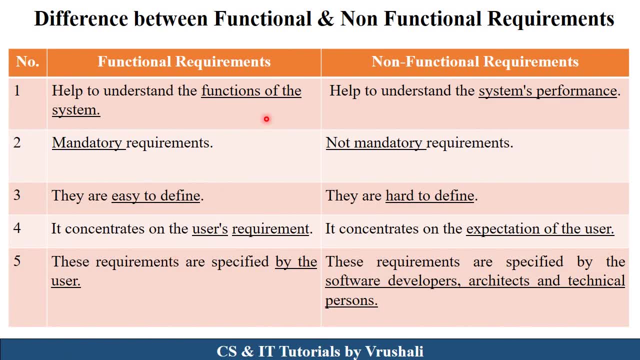 of software requirements. In software engineering, there are two types of requirement: functional and non-functional requirement. Let's see As per your exam point of view. this is one of the most important question, that is, difference between functional and non-functional requirement. 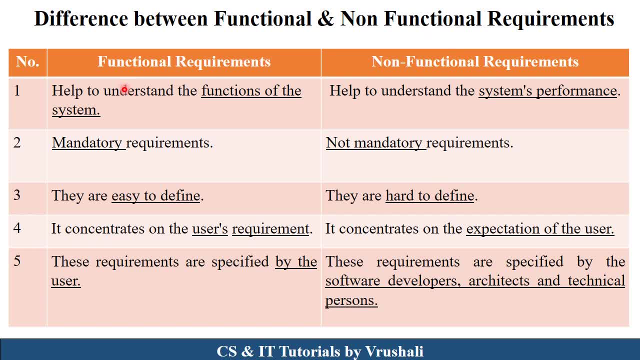 First we understand what exactly software requirement is. First we understand what exactly functional requirement is. Functional requirements help to understand function of the system. Means which type of features specification customer want. For example, customer want video call, audio call, chatting, this kind of features. So all the features related requirement. 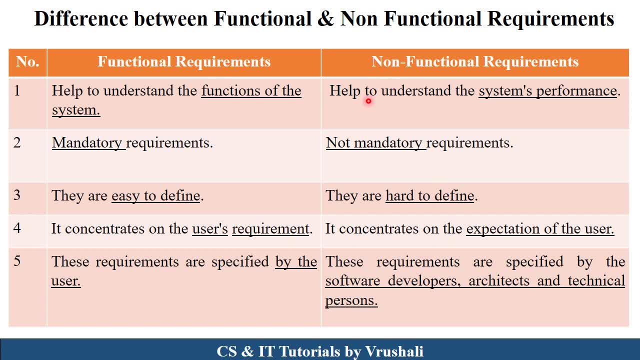 are called as functional requirement, But non-functional requirement help to understand the system. performance Means after developing how your product will work, their accuracy, their quality, their cost, their performance. So these are the two type of requirement that are called as non-functional requirement. so functional requirement based on the features. 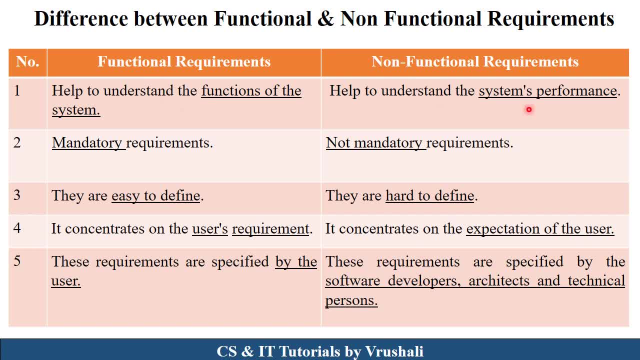 of the system and non-functional requirement based on the system performance. functional requirements are the mandatory requirement. non-functional requirements are the not mandatory because it depend on the functional requirement. functional requirements are very easy to define. user directly communicate with the project head and confirm their all the requirements. right, but non-functional. 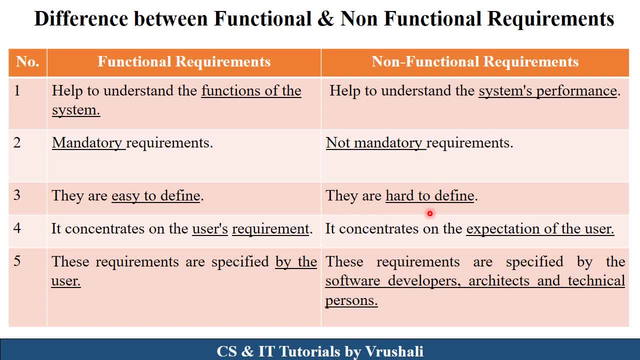 Functional requirements are very hard to define because it depends on the performance. Functional requirements are concentrated on the user's requirement, but non-functional requirements are the expectation of the user. what exactly user want, which type of performance they want? right? Functional requirements are specified by the user. non-functional requirements are specified. 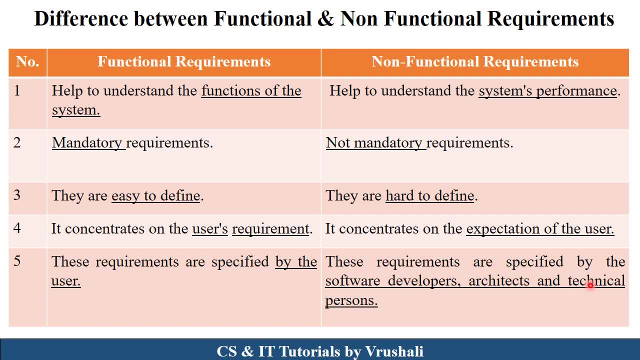 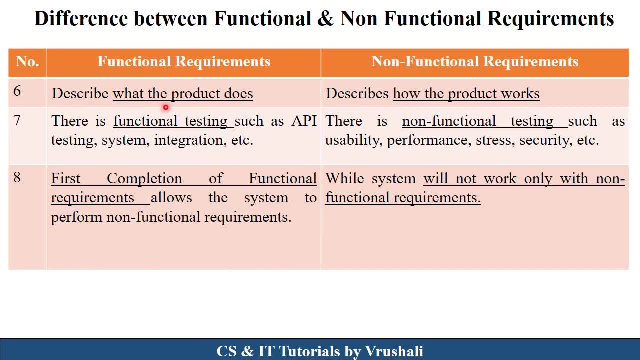 by software developer, software architect and the technical person. They handle performance of the system. In functional requirement describe what the product does, which type of features and function included in the particular product. But non-functional requirement means how the product work, their accuracy and their quality. 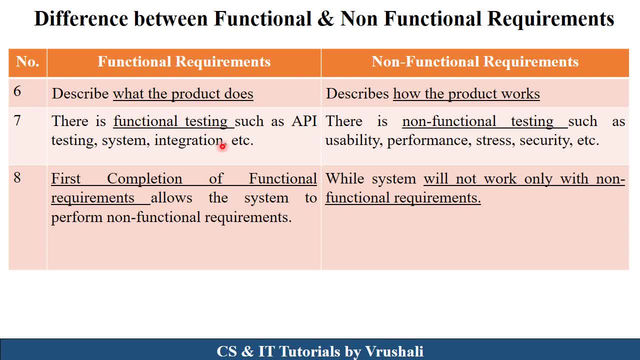 In functional requirement: functional testing have performed, which perform API testing system integration testing. Non-functional requirement: non-functional testing have performed which is related to the user. It is check that the particular product usable to the customer or not their performance. 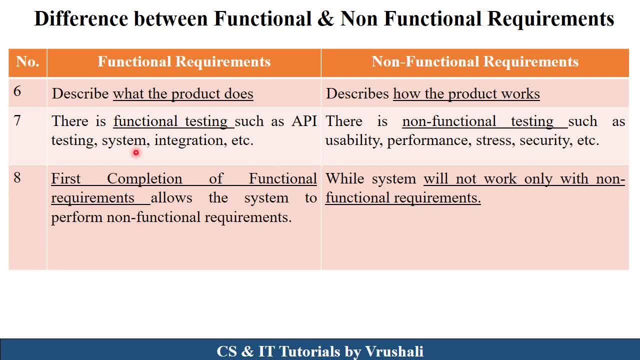 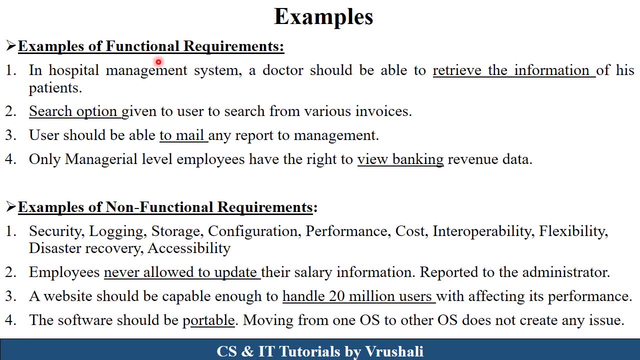 their stress and security related issues. So basically, first you need to complete functional requirements, then you need to complete non-functional requirements. Clear Next. Now here are some examples of functional requirements. Example of functional requirement: first, in hospital management system, doctor should. 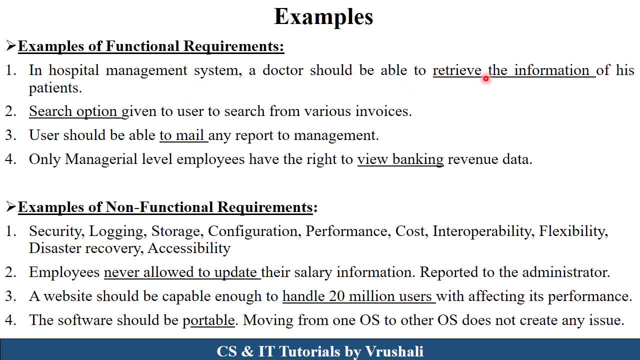 be able to retrieve the information of the patient, So retrieve- this is one of the feature- means to insert data, update data, delete data, retrieve data. So these all the features, these are the functional requirements. Then search option: to search a particular contact. to search a particular name. 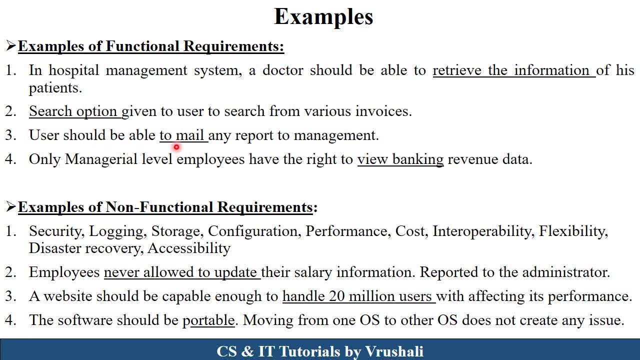 So searching is also one of the feature. Then user should be able to mail any report to the management In Gmail. there are mailing system is there, So this is also one of the feature. and only managerial level employee have to write to view banking revenue data means all the authentication related. which kind of person? 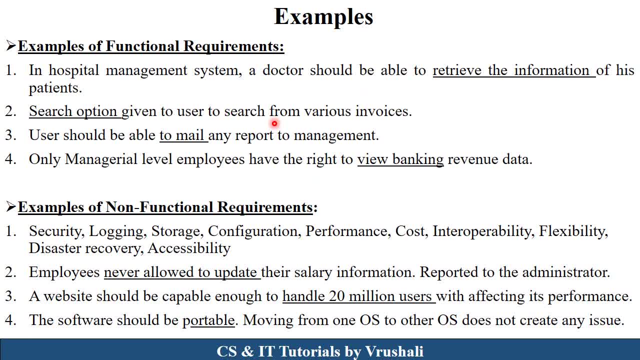 view which kind of information. So these all are the functional requirements. The examples of non-functional requirement means performance of the system, like security, logging, storage, configuration, performance, cost related requirement, then a flexibility, then recovery related, and accessibility and interoperability. this all are the performance. 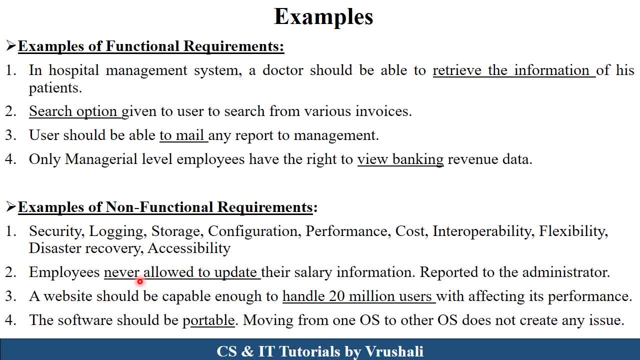 related requirements. Let's take a example. suppose employee never allowed to update their salary information, So there is a issue in performance right. The next one is a website should be capable enough to handle 20 million users with affecting it performance. Suppose a particular website. there are 20 million users are handle this website at the 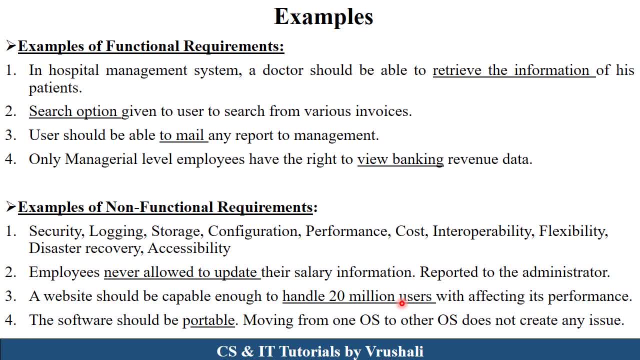 same time. So what was the performance? This is called as non-functional requirement. The next one is a portability issue. Suppose a particular product Work on Windows operating system and which is also work on Linux operating system means the particular product is portable, right? 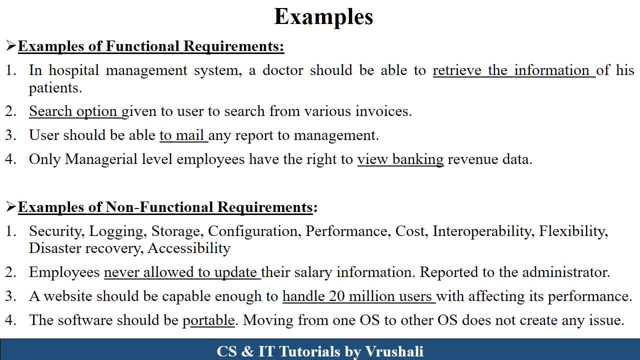 So these are the all are the non-functional requirement which is related to the performance. All about functional and non-functional requirement. Keep learning, Thank you.